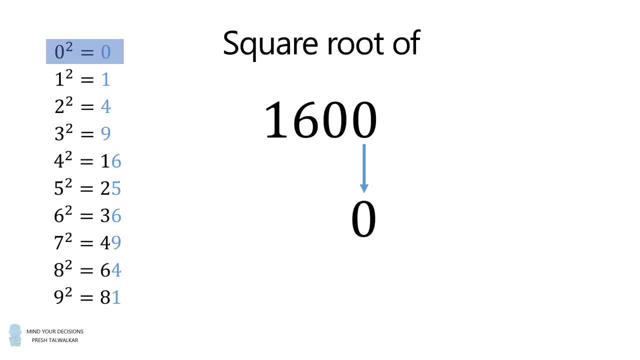 So we put a 0 over here. Then we cross out the hundreds and units digits. We're left with the number 16.. We now want to find the square that's closest to 16 without exceeding 16.. In this case, 4 squared is equal to 16 exactly. 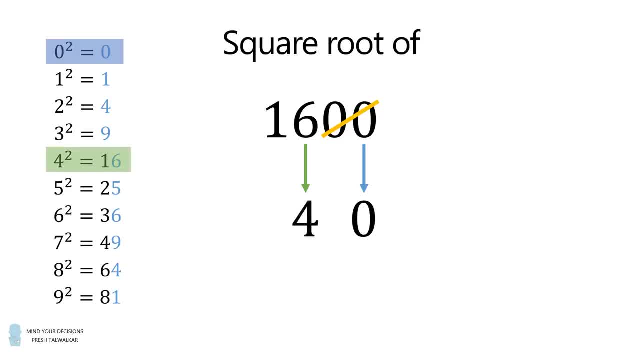 So we will write the digit 4 here. Thus the answer is equal to 40.. Now, this was a simple example. You probably could have calculated it without this method, But this method will show its value in more difficult examples, So let's go ahead with another example. 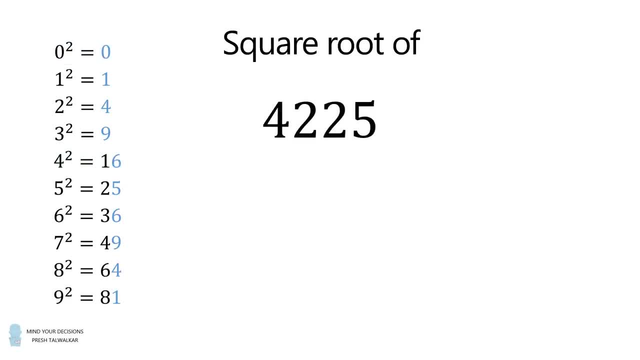 Let's calculate the square root of 4225.. The last digit is 5.. And that corresponds to the last digit of 5 squared, which is equal to 25.. So we write the digit 5 here. We then cross out the last two digits. 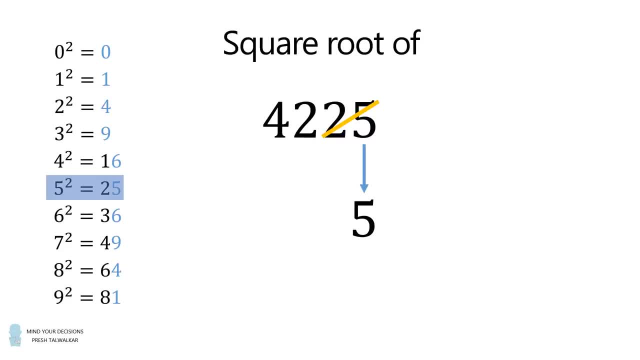 We now want the square that's closest to 42 without going over, So that will be 6 squared, which is equal to 36.. So we write a 6 over here. Thus the square root of 4225 is equal to 65.. 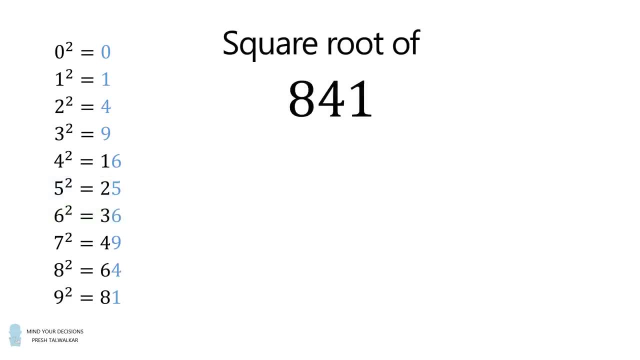 Now let's go to a little more complicated example. Let's calculate the square root of 841.. The last digit is 1., And that could either correspond to 1 squared, which ends in a 1., Or it could correspond to 9 squared, which ends in a 1 as well. 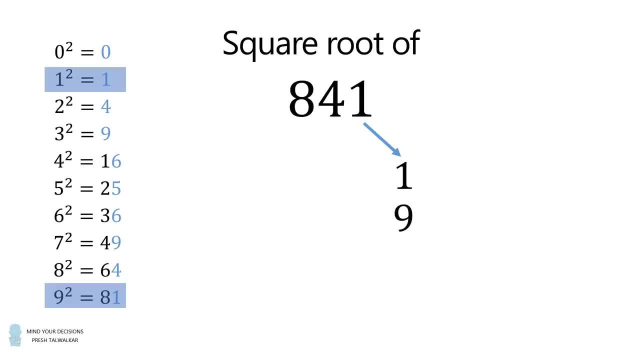 So we have two options of 1 and 9.. We'll sort this out in a little bit. We'll continue by crossing out the last two digits. Now we want the square that's closest to 8 without going over. So this will be 2 squared, which is equal to 4.. 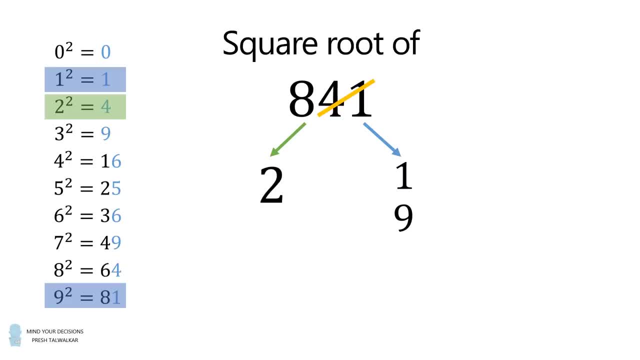 So we write a 2 here. So now we need to go to two options. We either have: 841 is equal to 21 squared, or 29 squared. To distinguish between the two, we'll use a genius method. We will calculate the square of 25, which is in between 21 and 29.. 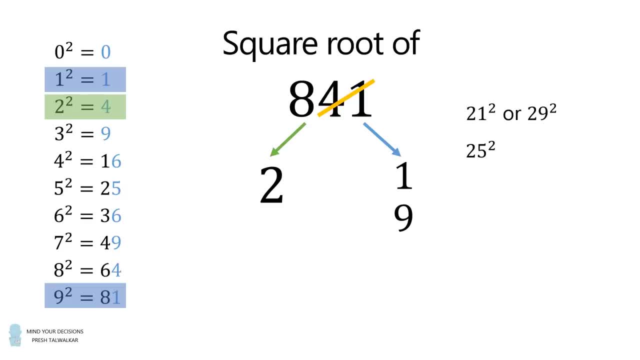 So there's a trick to calculating the square of a number that ends in 5.. You take the part of the number that's not 5,, in this case 2, and you multiply it by one more than itself. So we take 2 multiplied by 3, which is equal to 6.. 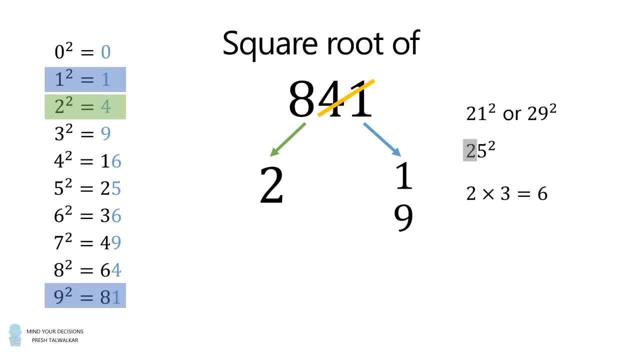 Then you append a 25.. So 25 squared is equal to 625.. Notice, 625 is smaller than 841.. So 25 squared is too little. So it must actually be the case that 841 is equal to 29 squared. 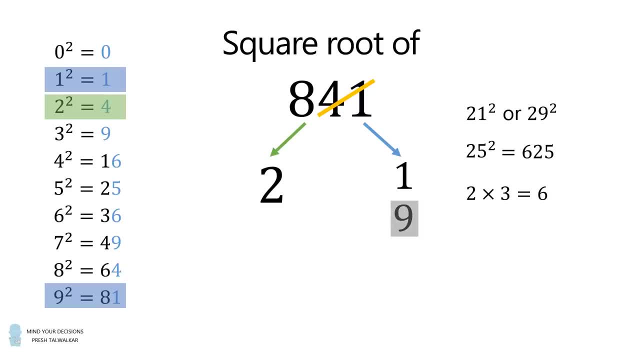 Thus we take the larger option of 9.. So the square root of 841 is equal to 29.. This may sound a little complicated, but it'll get easier as we work through more examples. Let's now calculate the square root of 39, 69.. 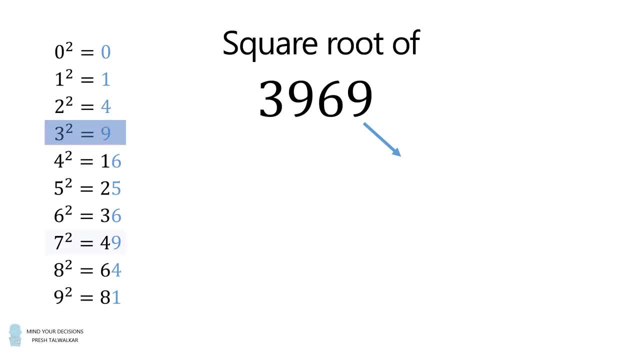 We go to the last digit of 9, and we know that it's either 3 or 7.. We then cross out the last two digits and we look for the square that's closest to 39. without going over, This will be 6 squared, which is equal to 36.. 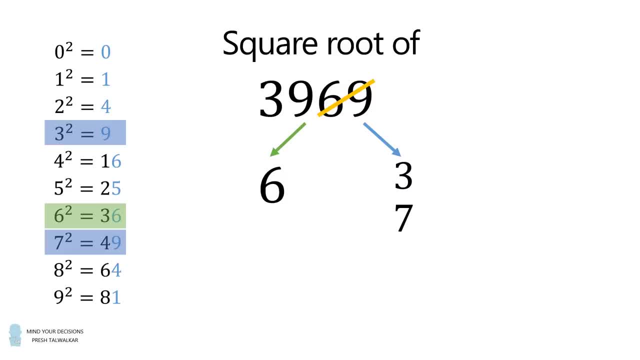 So we now need to differentiate between 63 and 67.. We will calculate the square of 65, which is right in the middle. So we take 6 and multiply it by one more than itself to get 42.. Now notice, if we have 42,, 25,. 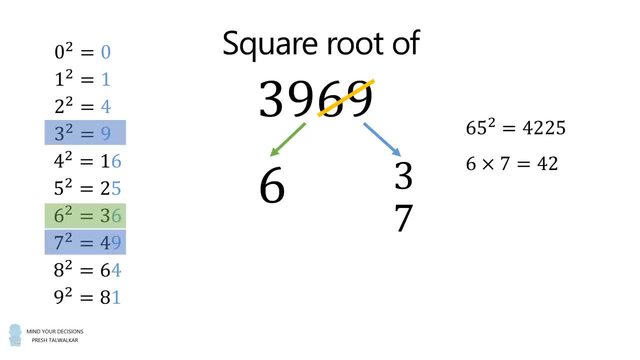 that'll be larger than 39, 69.. So 65 squared is too large, So it must instead be equal to 63 squared. So thus we know the square root of 39, 69 is equal to 63.. Wow. 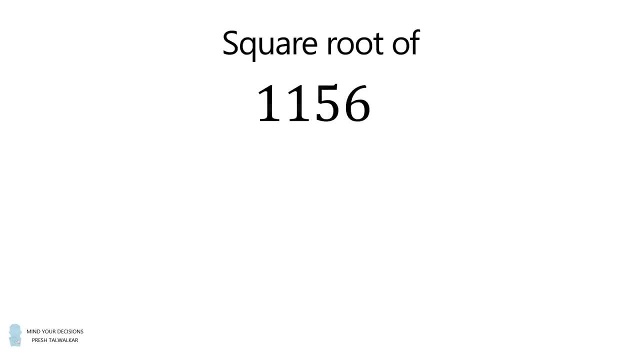 Let's now calculate the square root of 11, 56.. From the last digit we know the options are either 4 or 6.. We then cross out the last two digits. We look for the square closest to 39.. We look for the square closest to 11, without going over. 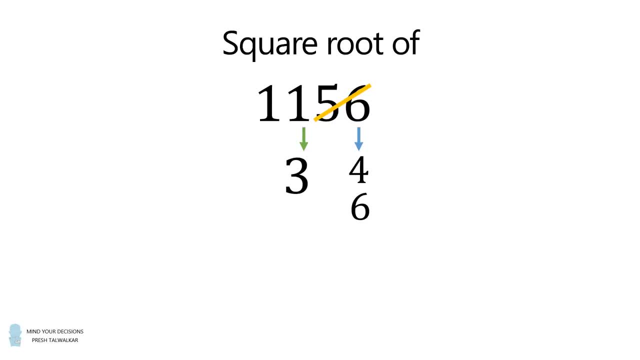 which will be 3.. We now need to differentiate between 34 and 36.. So we take 3 multiplied by one more than itself, which is 12.. Now 12 is larger than 11, so we need to pick the smaller option of 4.. 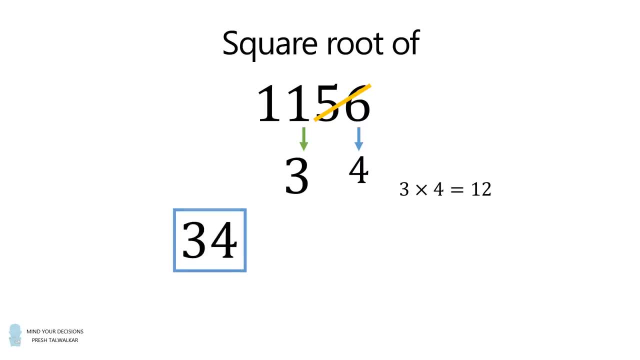 Thus, the square root of 11, 56 is equal to 34.. We can adapt this solution to calculate the square root of 11.56.. This will be equal to 3.4.. Now let's calculate the square root of 16, 384.. 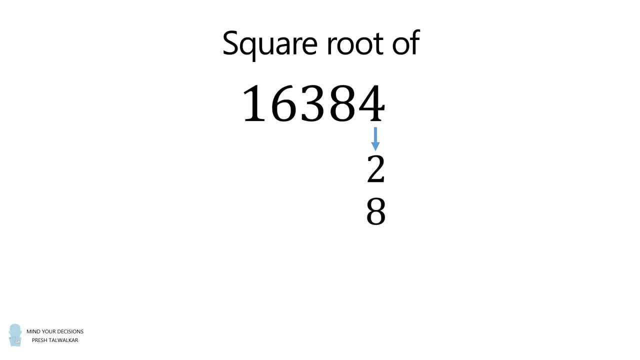 From the last digit. we know the two options are either 2 or 8.. Then we cross out the last two digits. We want the square that's closest to 163 without exceeding 163.. This will be 12 squared, which is 144.. 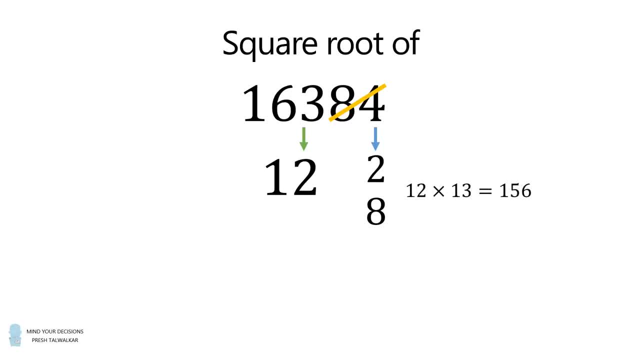 We now take 12 multiplied by one more than itself, which is 156.. Then we see that 156 is smaller than 163, so we take the larger option of 8.. Thus the square root of 16,384 is equal to 128.. 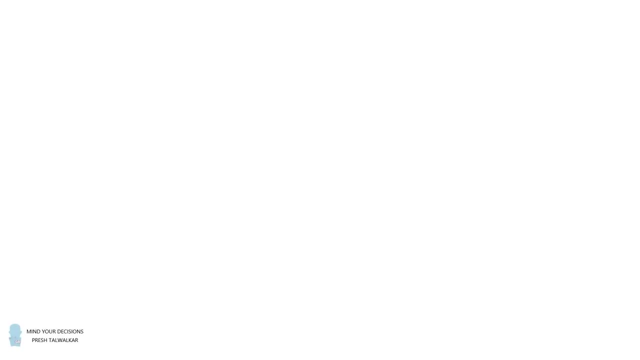 Wow. I will mention that you can also adapt this method to calculate the cube root of a number. You of course first have to memorize the cubes of the numbers from 0 to 9. Then the procedure is very similar. In fact it's even easier, because each of the last digits is different. 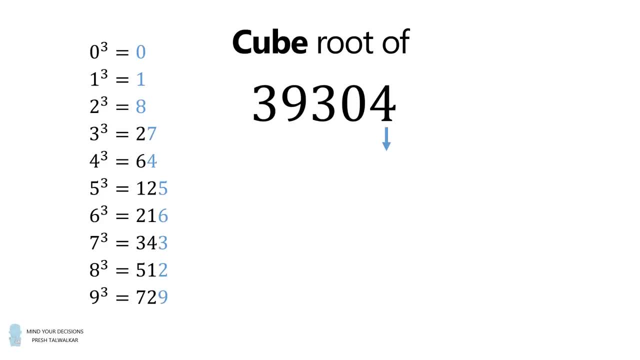 So we look for the cube whose last digit is equal to 4.. The only option is 4 cubed, which is equal to 64. So we put down a 4 here. We then cross out the last three digits. We look for the cube that's closest to 39 without going over. 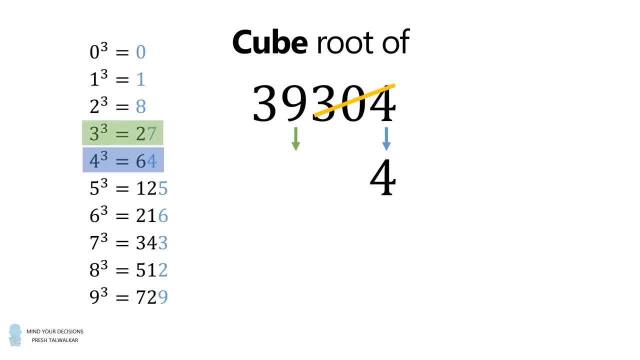 This will be equal to 3 cubed, which is 27.. So we put a 3 here. Thus, the cube root of 39,304 is equal to 34.. Amazing. Now, in the present day, we often take arithmetic for granted.